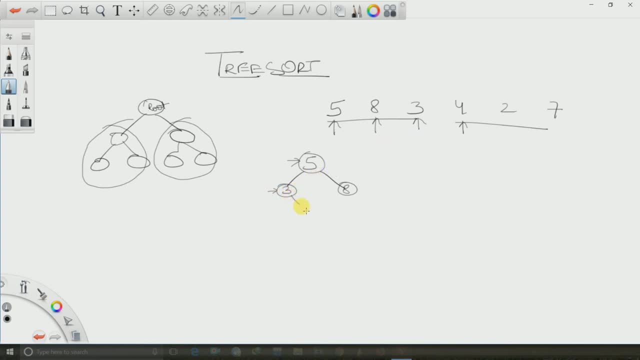 now four is greater than three, so you will go to its right child and you will insert here, since this is the open space. now you want to insert two. now again start scanning from five. so since five is greater than two, so two will will always be present in its left. 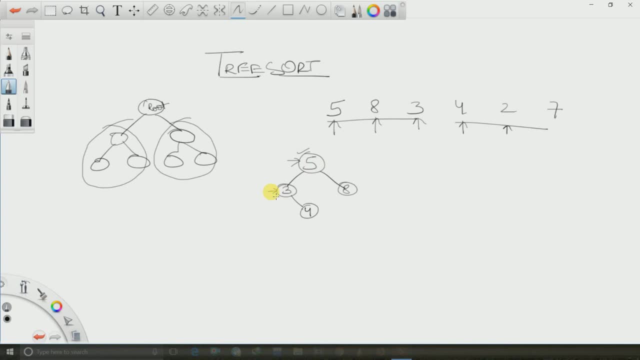 sub tree. so two, so you will go to the its left child. okay, now you will compare with three. so since three is greater than two, so two will go to its left child, and since left is empty, so you can insert it here. okay, two, now you go to seven. since five is less than seven, so seven will be present as its. 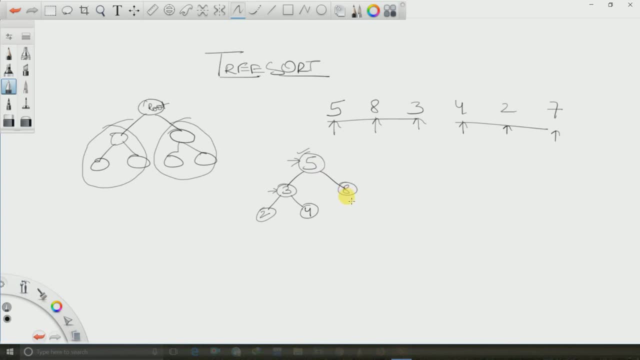 right child. so you go to eight, since eight is greater than seven. so seven will be present as its left child and it will be inserted here. so this is the binary search tree which you have found. okay, now for to see the element in the sorted order: what you. 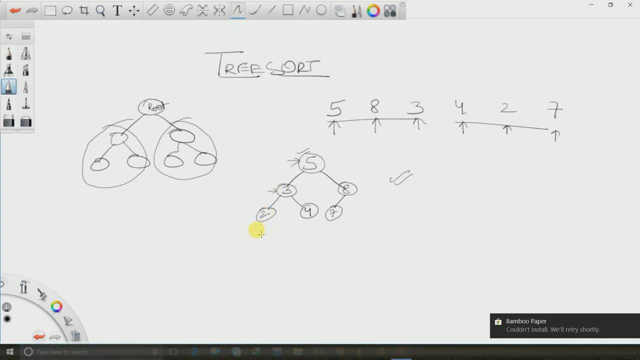 can do is just do the in order traversal. you know that in in order traversal, when you, when you traverse a node for the second time, you will print that node. so start scanning from five. okay, now you reach to. okay, so you will print as output after in order traversal as two, then after two. 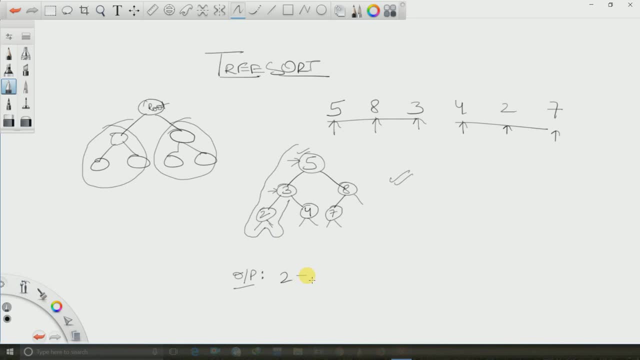 you will go to three, so you will print in three. after three you will go to four and you will print four and like this, you went to five. you will print five, then to seven and then eight. okay, this is how it is done. so this is basically tree sort, so you must be knowing this from. 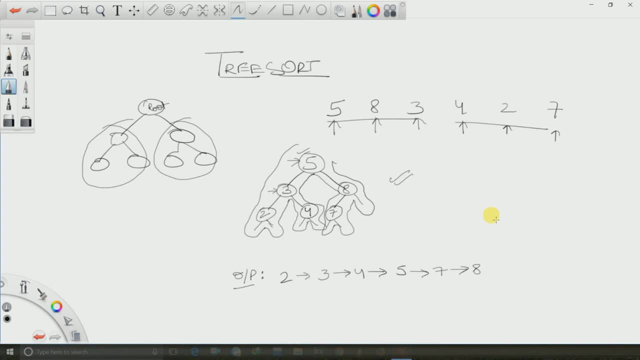 the very beginning, but only the name is given that sorting using a tree, so it is called as a tree sort. so I hope to see you in my next lecture and if you like this video, then please hit a like button and subscribe for more such videos. thank, you.